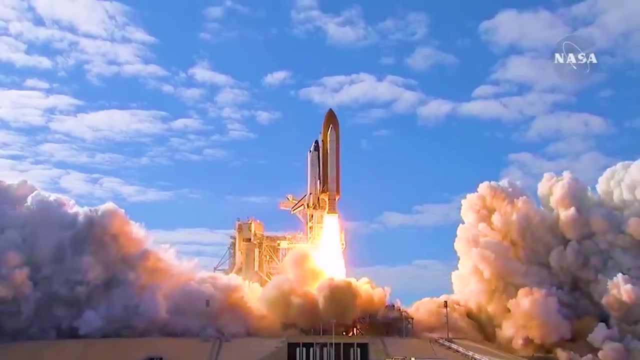 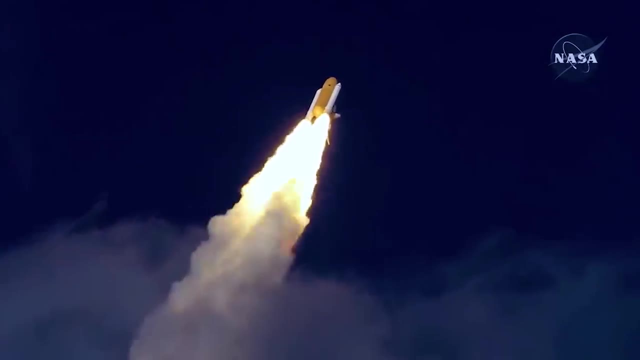 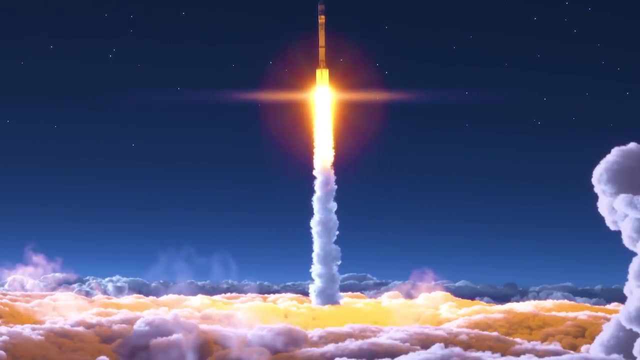 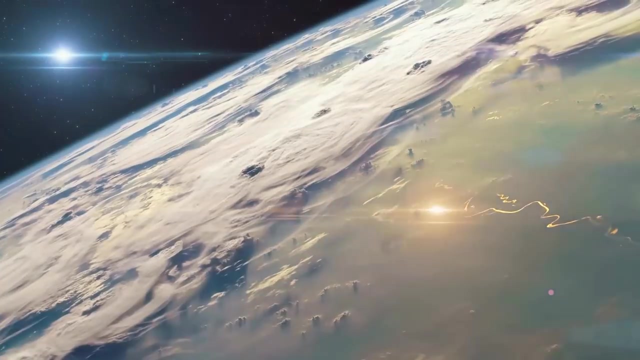 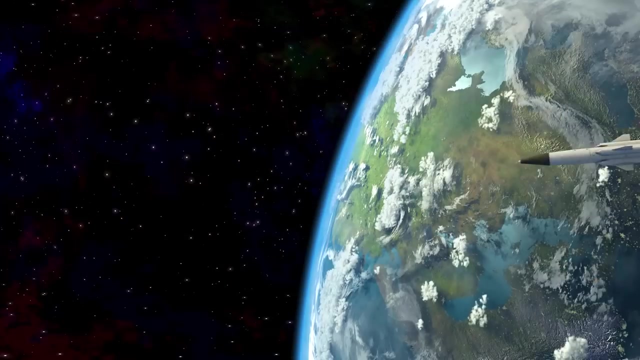 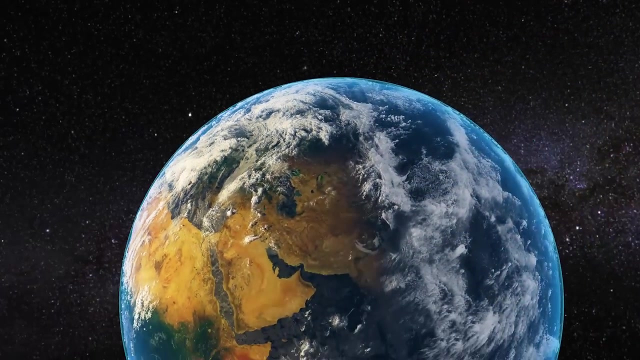 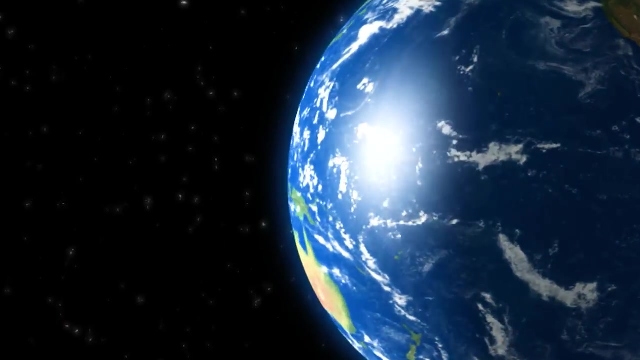 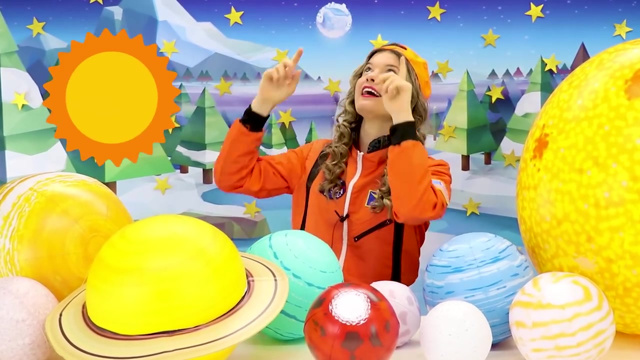 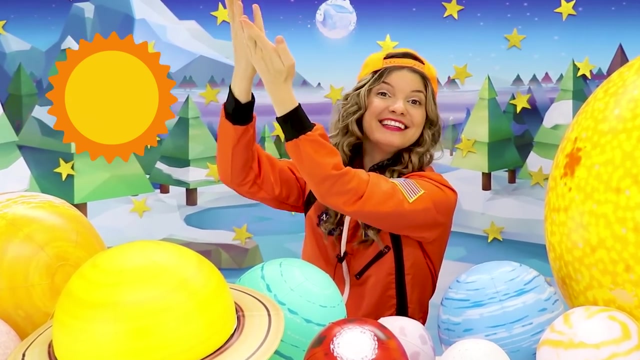 And liftoff. The rocket goes up towards the sky. The rocket leaves Earth's atmosphere and goes into space. And this is our planet Earth, Cool huh. When you see the Sun up in the sky, it looks really small. You can almost hold it with your hands. 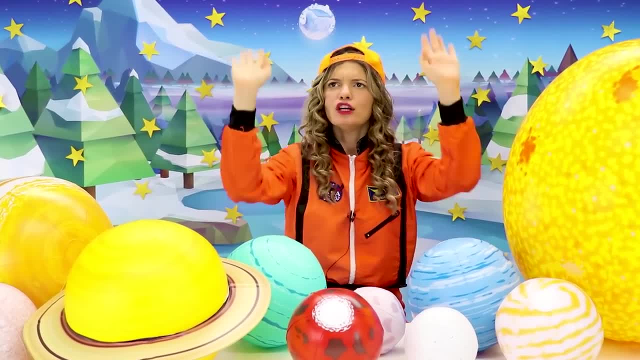 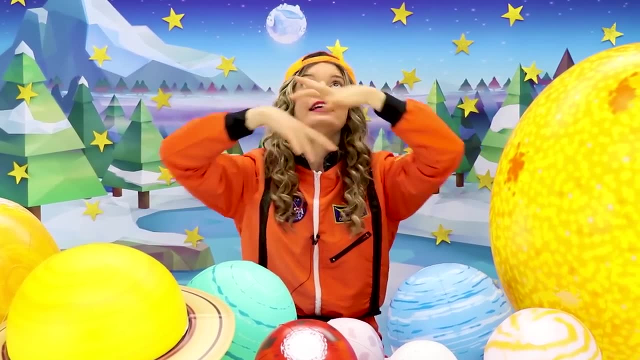 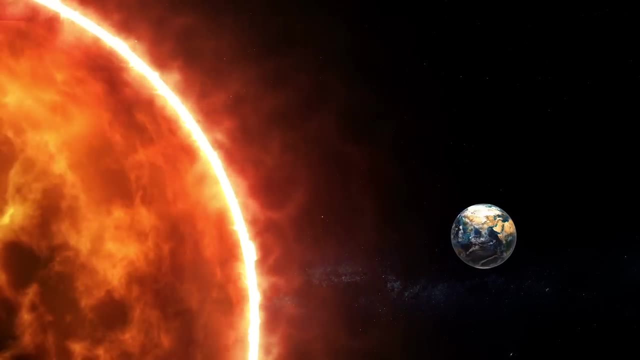 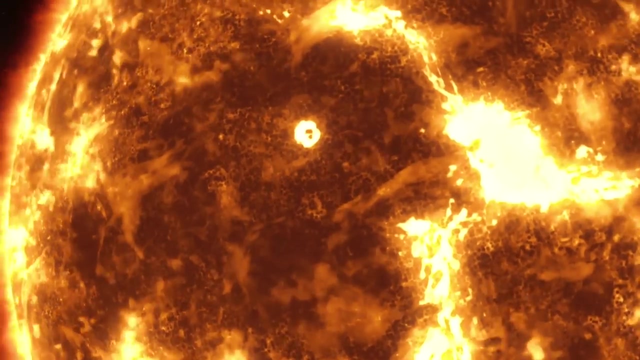 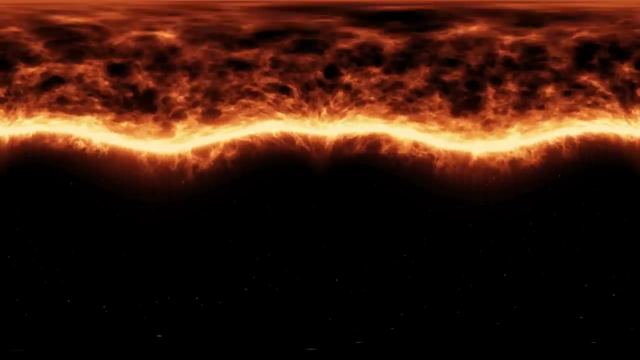 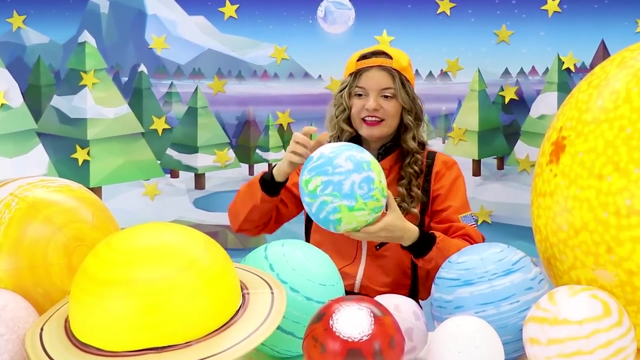 But it only looks small because it's so far away from us. In reality, the Sun is huge. It's much bigger than Earth And it is very, very big, Very, very hot. Our planet Earth likes to get warm, So it goes around the Sun to get warm on all sides. 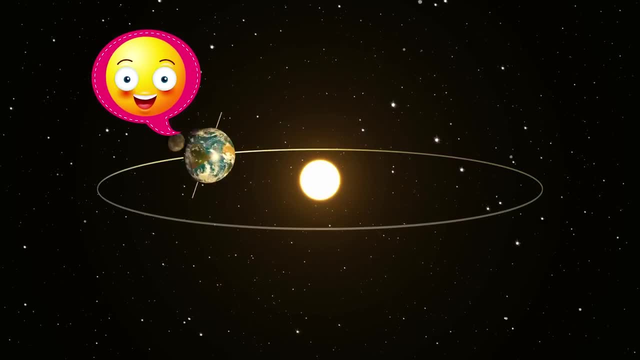 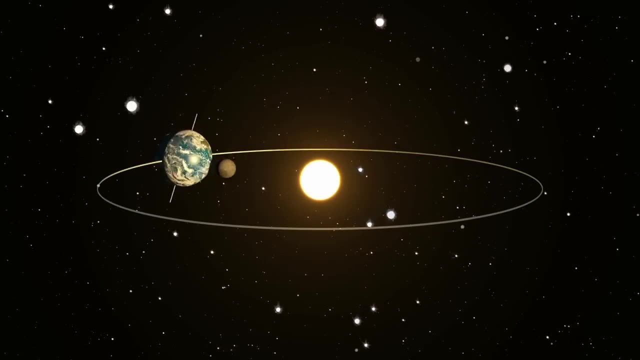 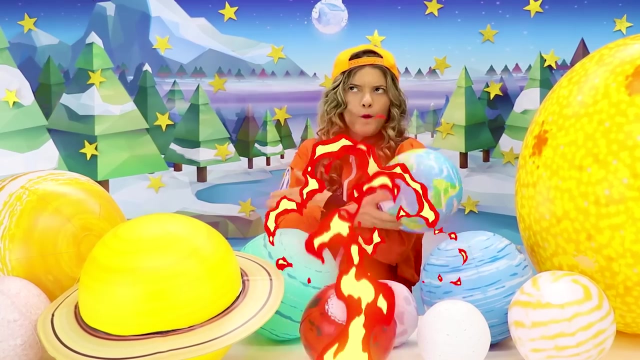 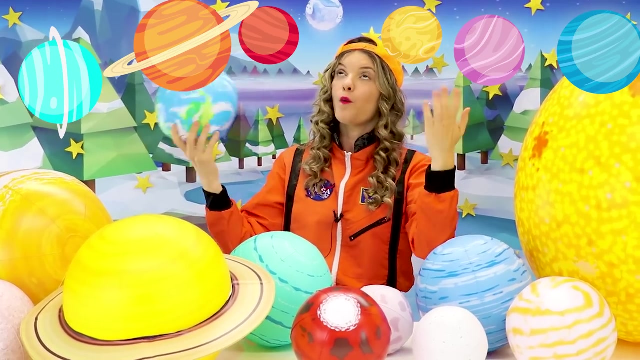 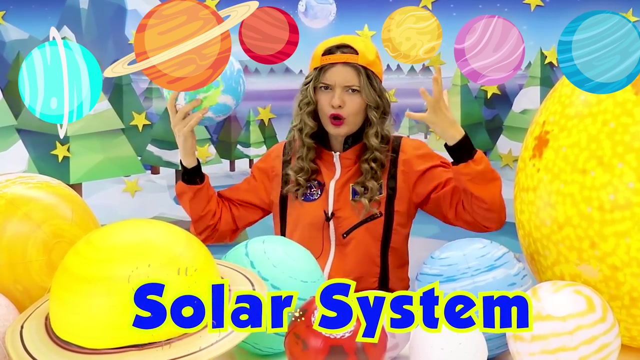 Like this. Oooh, It's so nice and toasty here, We like it. But Earth is not the only planet that likes to feel warm. We have several other planets that want to get warmed up by our Sun, And those planets are part of our solar system. 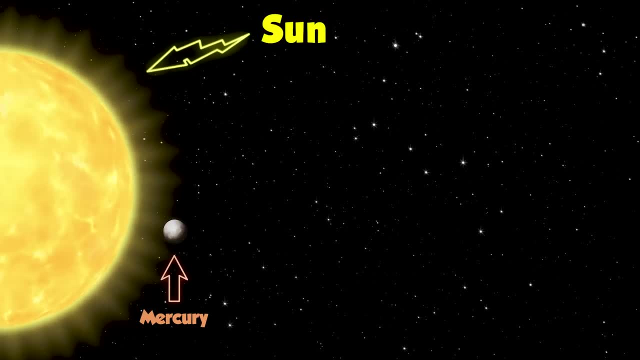 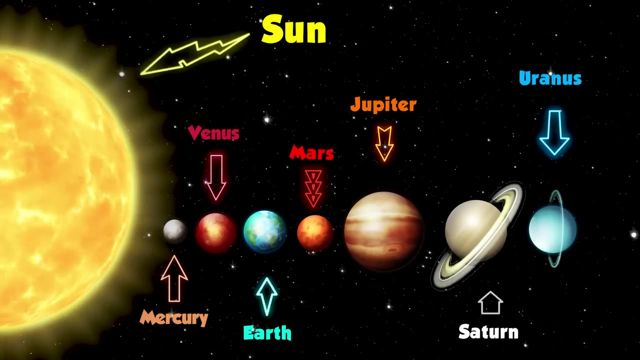 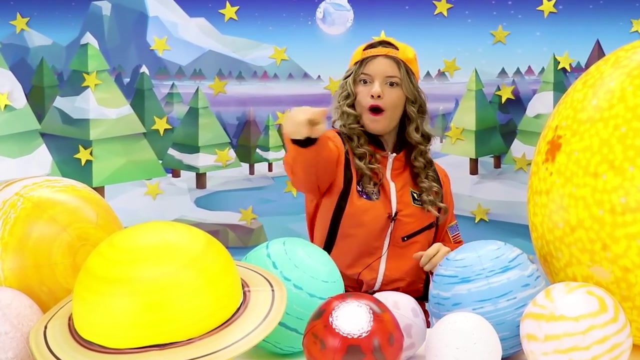 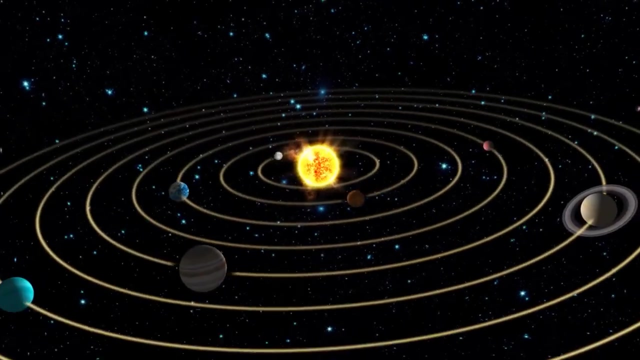 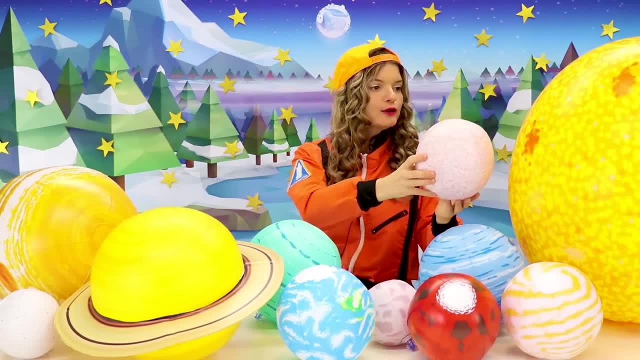 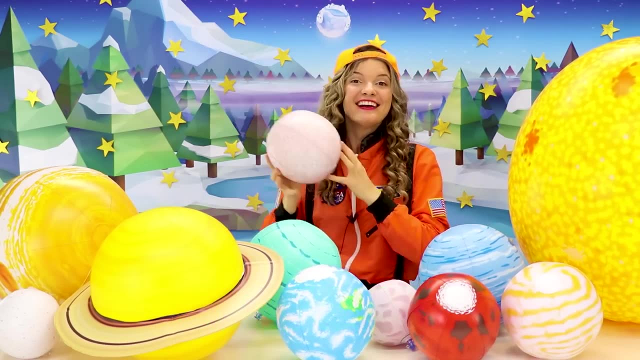 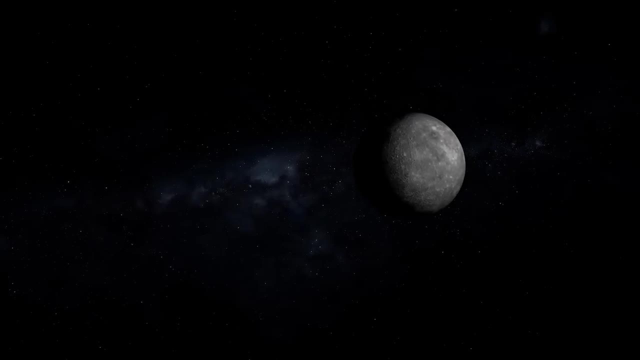 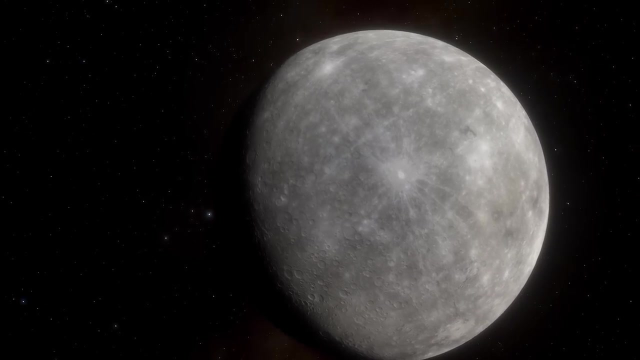 Hey, Hey, And the planet closest to the Sun is called Whoop, Whoop, Mur-cur-y. Ha ha, Can you say that, Muh Cur Ruy? Good job, This is what Mercury looks like. 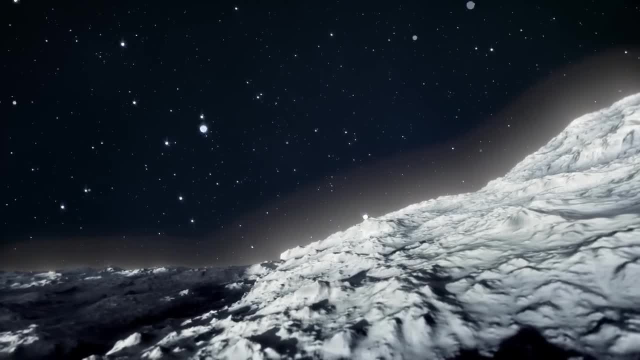 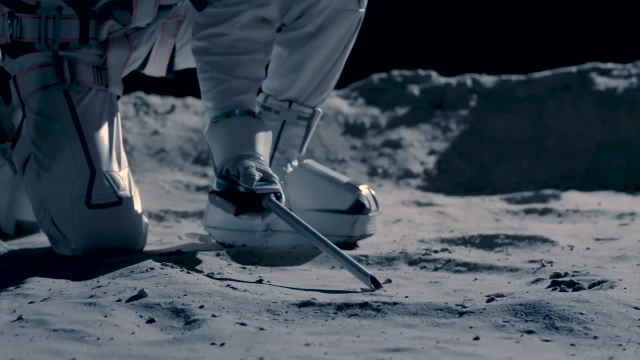 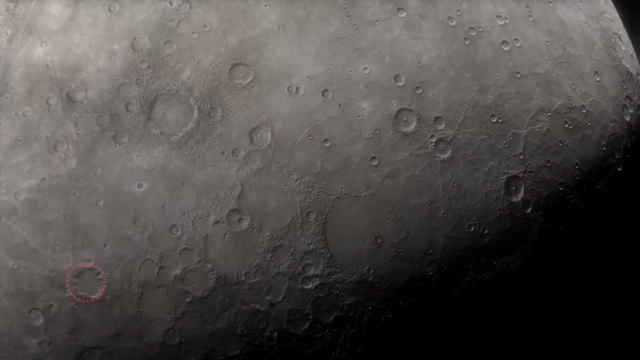 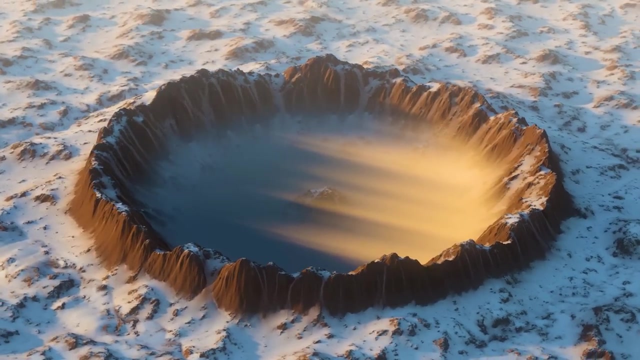 Mercury has a rocky surface on its outer surface. Vocêsfpsem unavogados. This surface it has is called the Cretaceous Strait, on which someone could walk, and the surface has a lot of these circles called craters. craters are created when huge space rocks hit the planet. 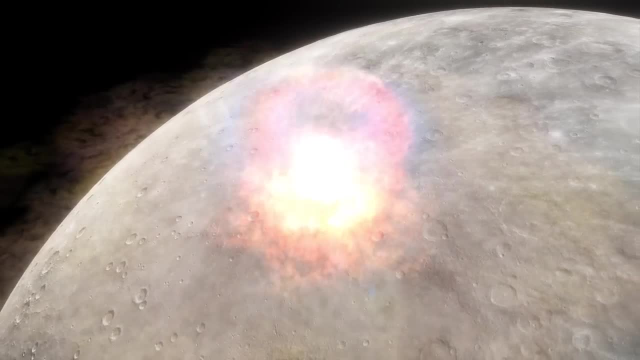 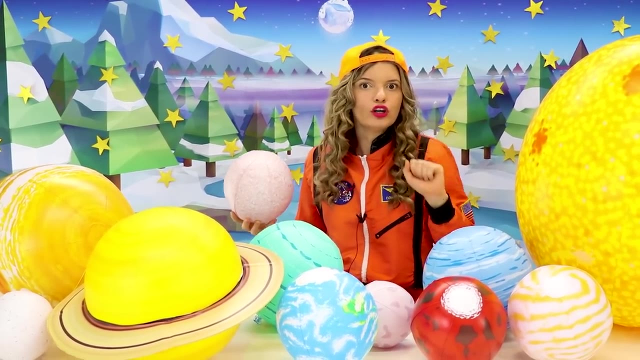 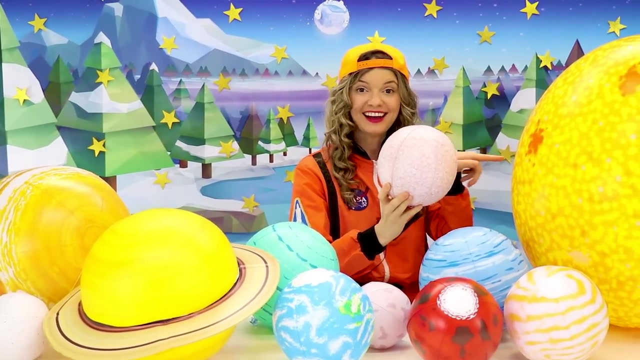 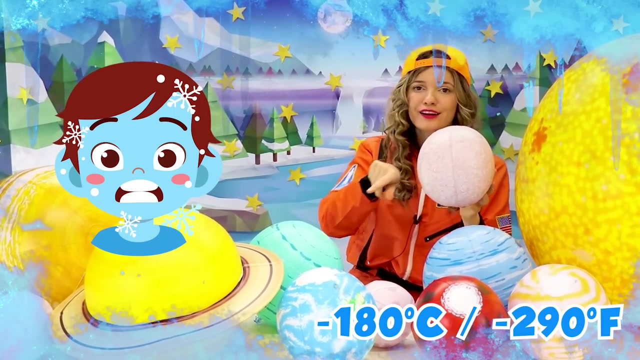 the weather on mercury is really wild. it goes from being extremely, extremely hot when it's facing the Sun to be really, really cold when it's in the dark. so you know what: you and I, we would not be able to see the sun when it's really really. 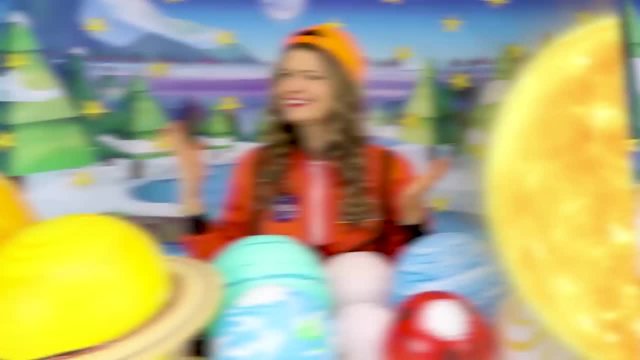 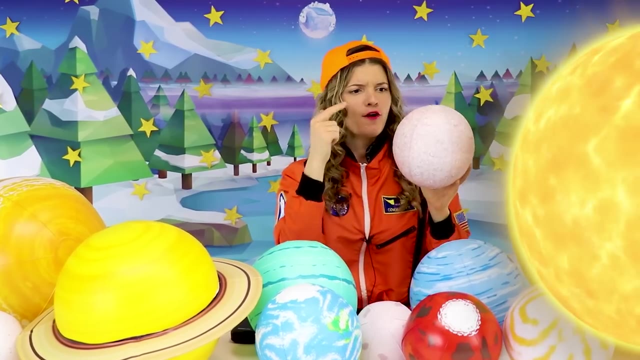 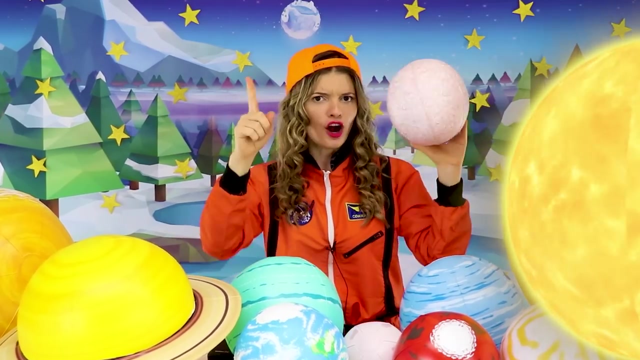 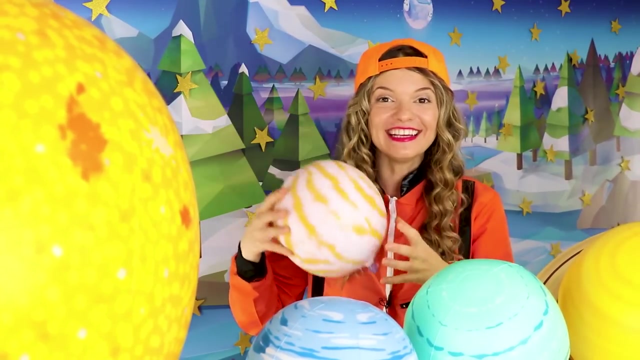 hot. we would not survive on mercury. so if this is our Sun and right next to it we have mercury, then over here comes a planet called Venus is a beautiful name for a very stormy and wild planet. Venus is a beautiful name for a very stormy and wild planet. 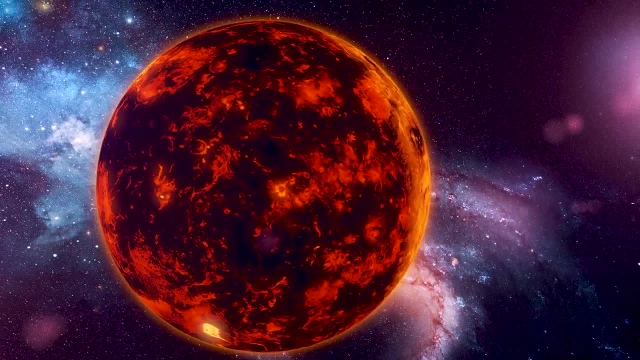 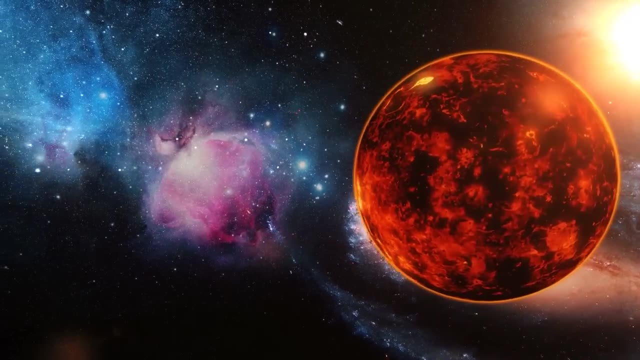 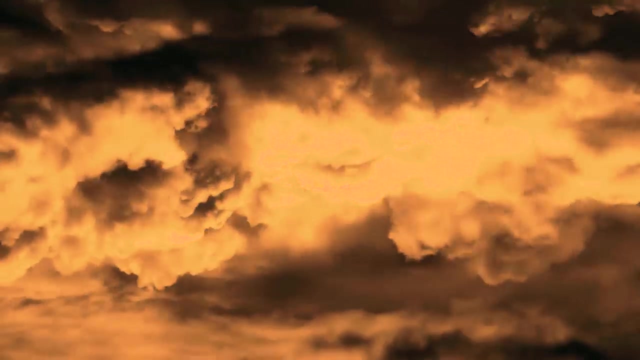 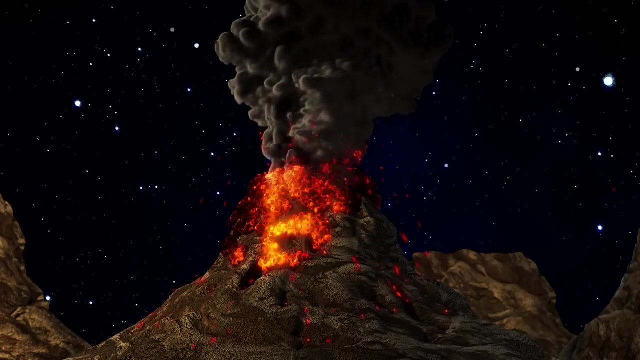 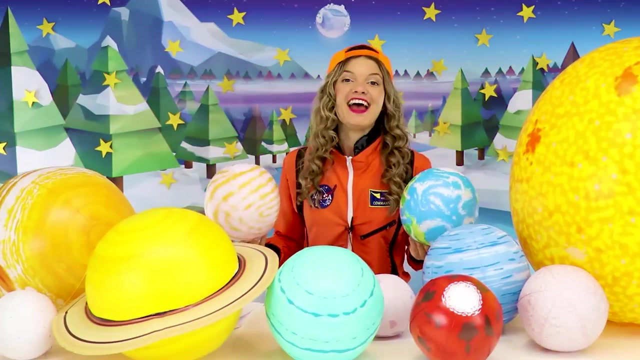 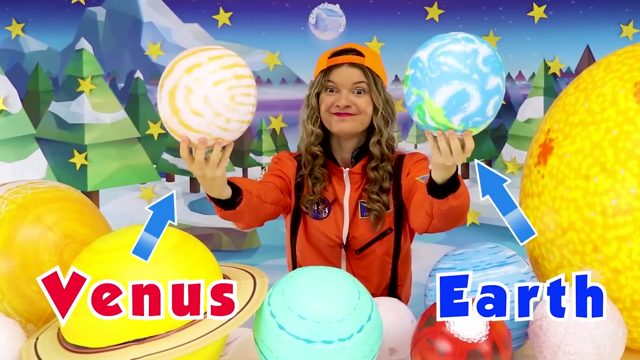 Venus is the hottest planet in our solar system. on this planet, there are very strong storms, thousands of volcanoes, thousands of volcanoes. and even though Venus is similar in size to Earth, see, we would not be able to. and even though Venus is similar in size to Earth, see, we would not be able to. 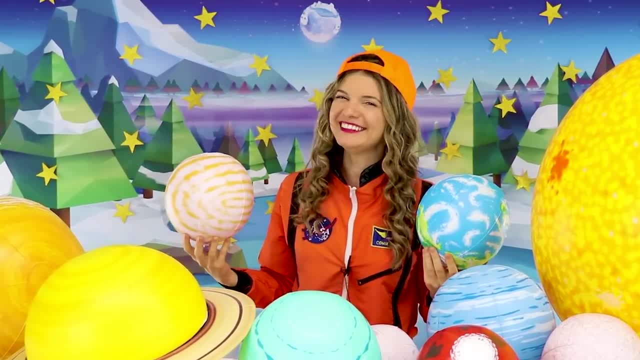 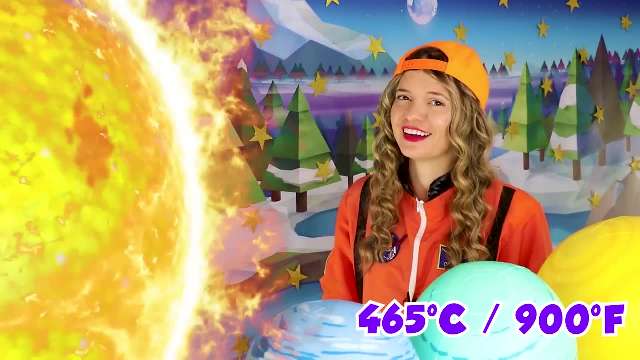 live on Venus because, firstly, it is super duper, duper hot there, too hot for see. we would not be able to live on Venus because, firstly, it is super duper, duper hot there, too hot for us, but also the surface pressure is so so us, but also the surface pressure is so, so so. 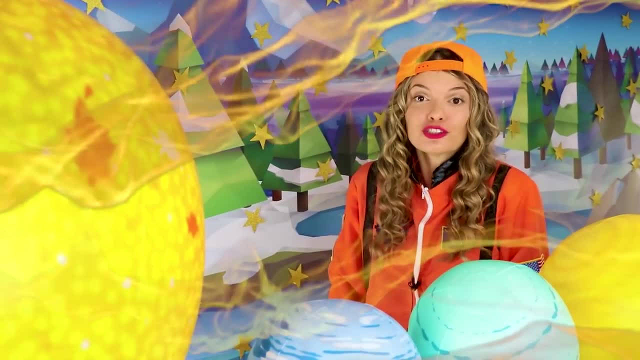 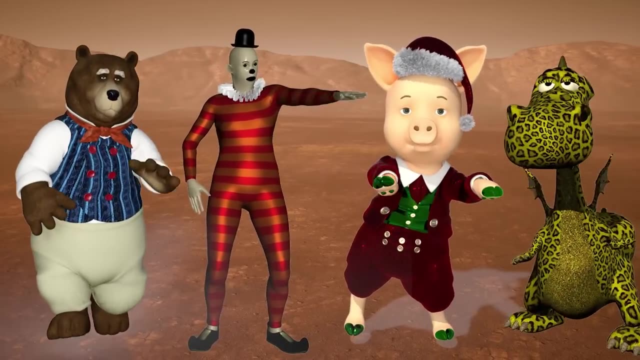 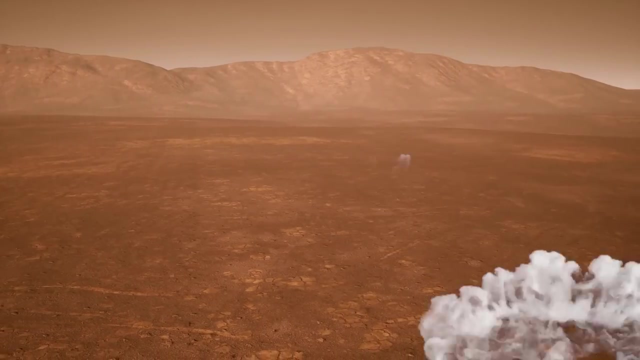 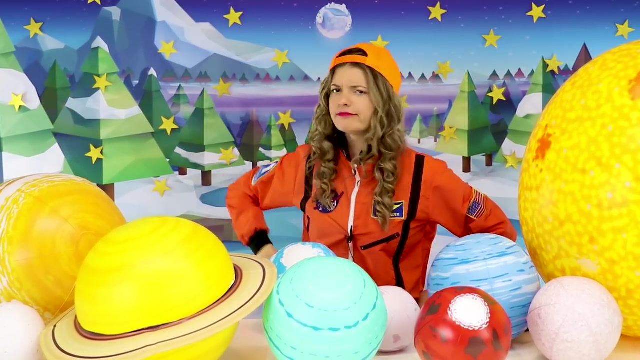 us, but also, the surface pressure is so, so, so strong that anybody who tries to go there strong that anybody who tries to go there strong that anybody who tries to go there would immediately get crushed. but that's would immediately get crushed. but that's would immediately get crushed. but that's alright, we don't need you, Venus, we have. 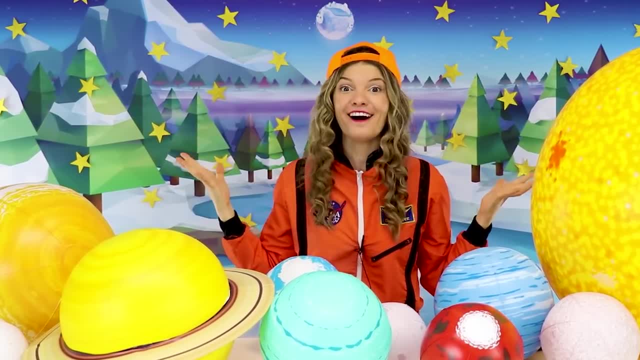 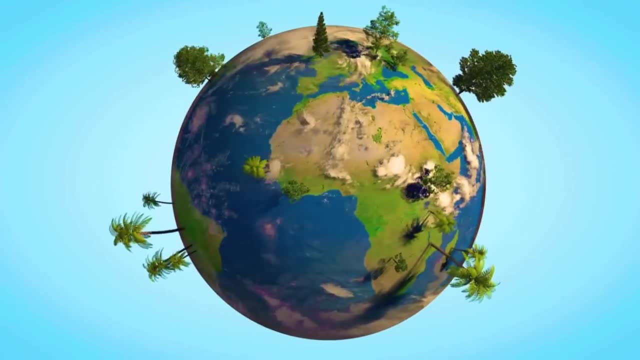 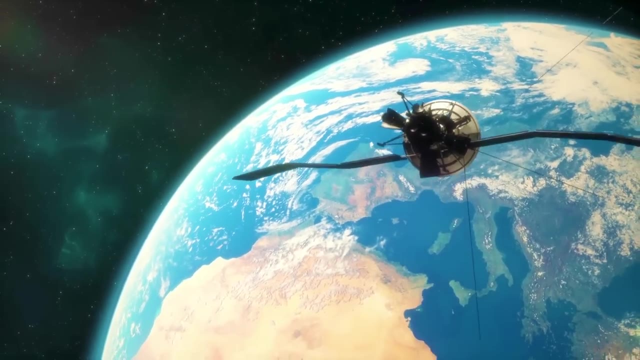 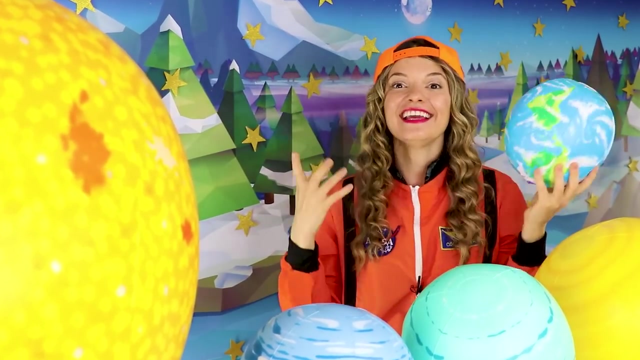 alright, we don't need you, Venus, we have. alright, we don't need you, Venus, we have the most amazing planet of all planet, the most amazing planet of all planet, the most amazing planet of all planet Earth. our planet is the only planet we know of. our planet is the only planet we know of. 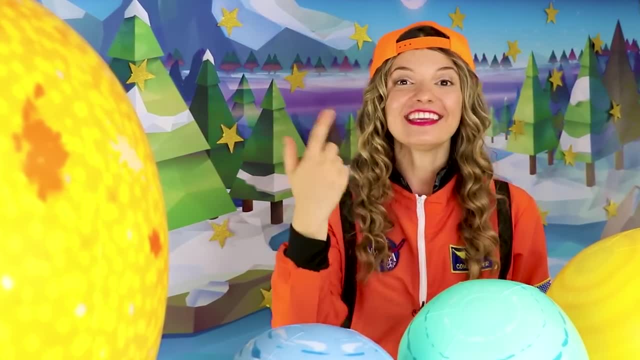 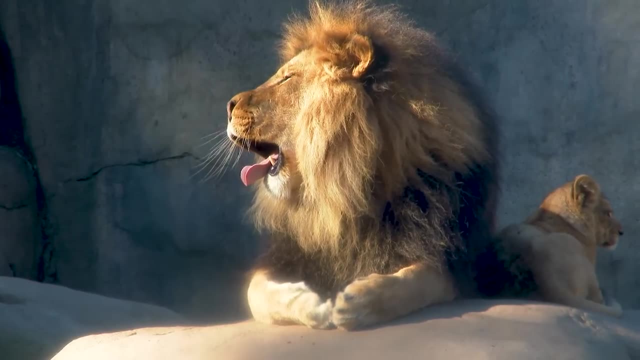 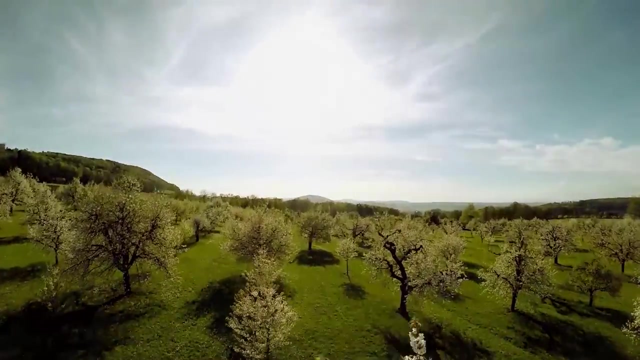 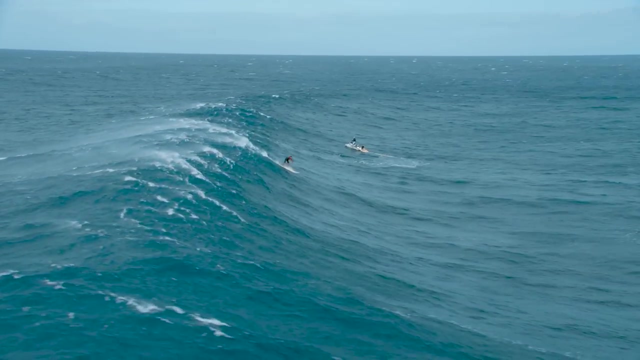 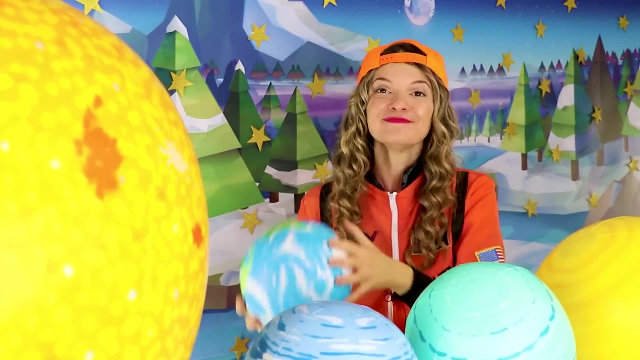 our planet is the only planet we know of to have life on it, to have life on it. to have life on it like you and I, and like animals or trees. earth is the only one and, and, and, and, and and. right next to us there's another, very 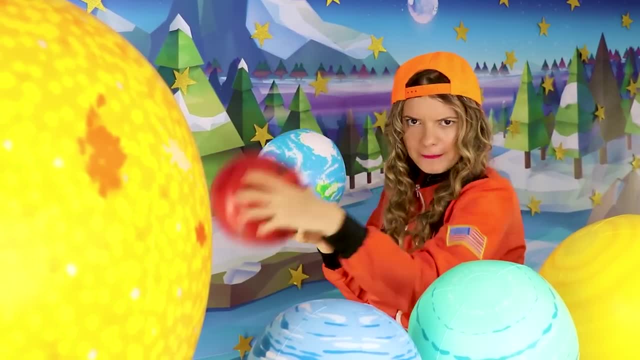 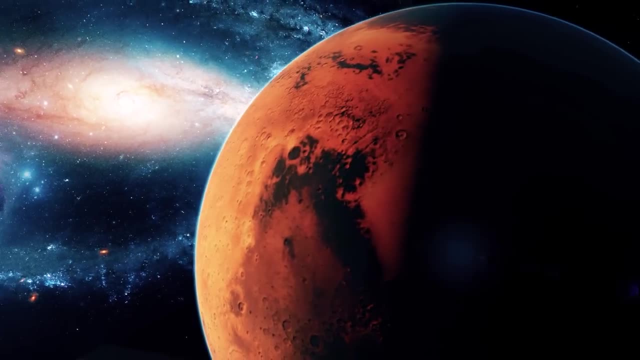 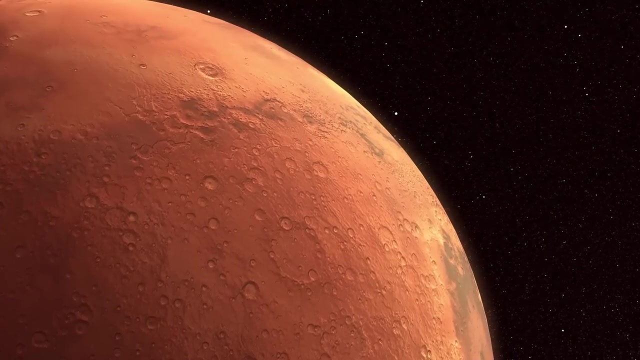 right next to us there's another very right next to us. there's another very interesting planet called planet Mars. interesting planet called planet Mars. interesting planet called planet Mars. Mars is sometimes called the red planet. Mars is sometimes called the red planet. Mars is sometimes called the red planet because of its color. 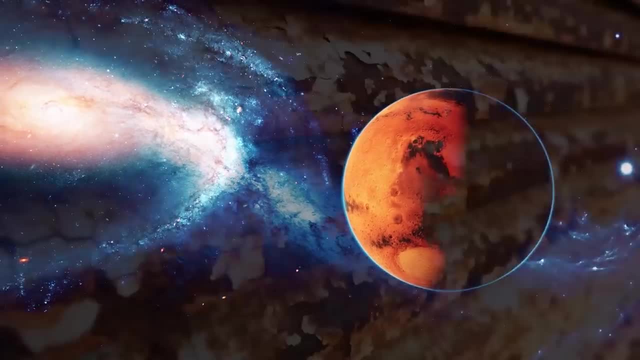 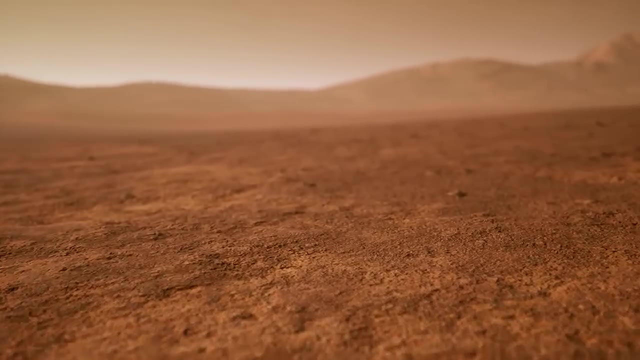 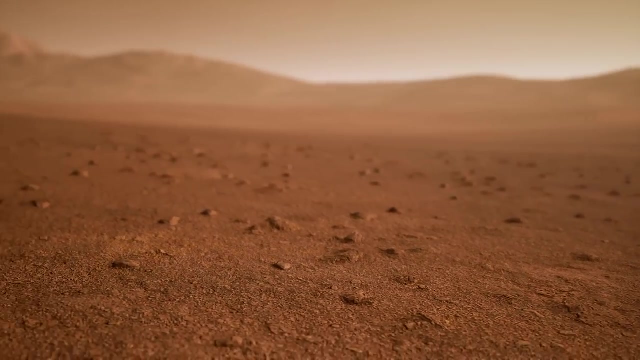 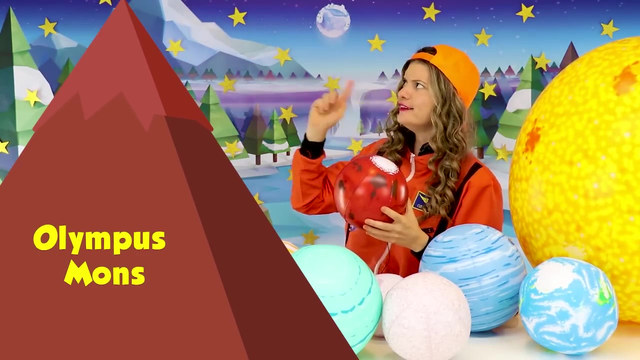 Mars gets this color from rust. Mars gets this color from rust. Mars gets this color from rust and Mars has a lot of rust in its rocky surface and Mars has a lot of rust in its rocky surface and Mars has a lot of rust in its rocky surface. on Mars there's a huge mountain called Olympus. 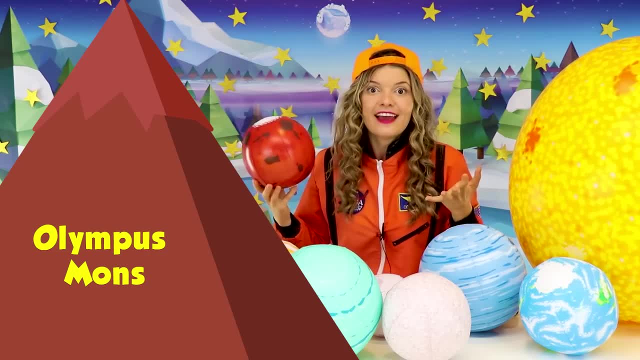 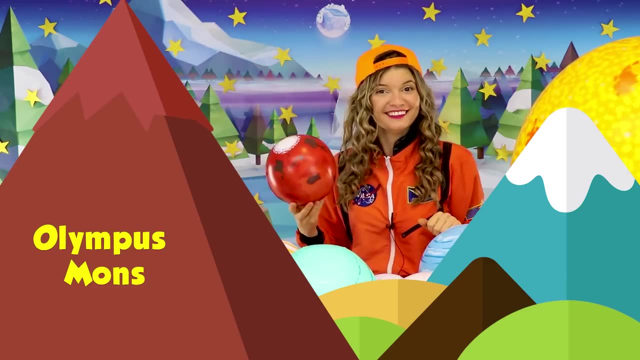 on Mars, there's a huge mountain called Olympus. on Mars, there's a huge mountain called Olympus, Mons. that mountain is taller than any mountain, Mons. that mountain is taller than any mountain Mons. that mountain is taller than any mountain that we have on beautiful earth. that we have on beautiful earth. 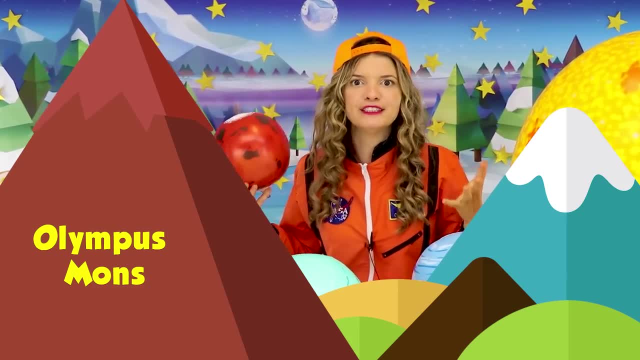 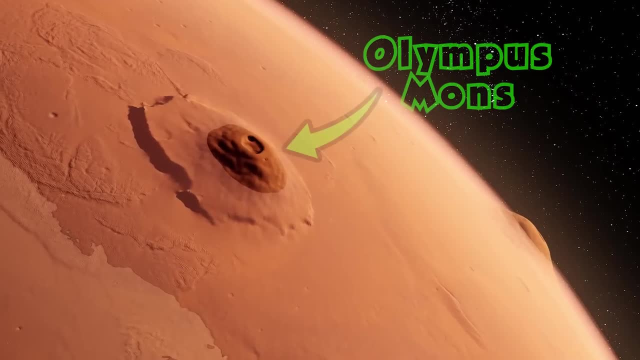 that we have on beautiful earth. oh, do you wanna see how olympus mons? oh, do you wanna see how olympus mons? oh, do you wanna see how olympus mons looks from space? looks from space, looks from space. me too, let's see. 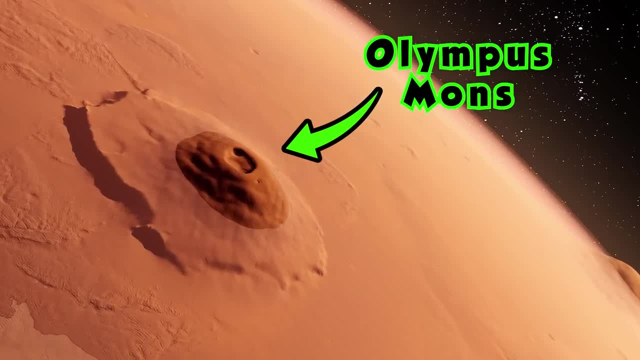 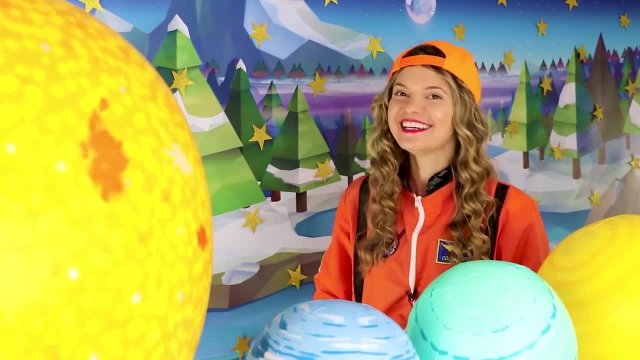 me too. let's see me too, let's see. this is olympus mons. and did you know that some years back? and did you know that some years back? and did you know that some years back, we sent a special. we sent a special, we sent a special robot to help us explore. 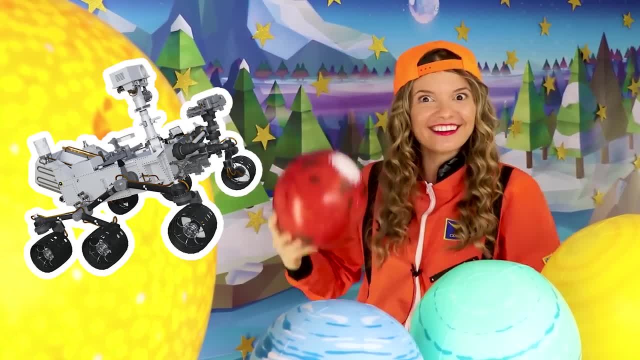 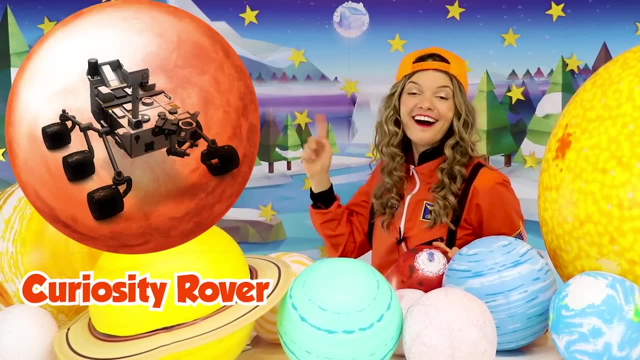 robot to help us explore, robot to help us explore mars, and that robot is still mars, and that robot is still mars, and that robot is still there, there, there, that's right, that's right, that's right. a rover called curiosity, a rover called curiosity, a rover called curiosity, was sent to mars to help us learn. 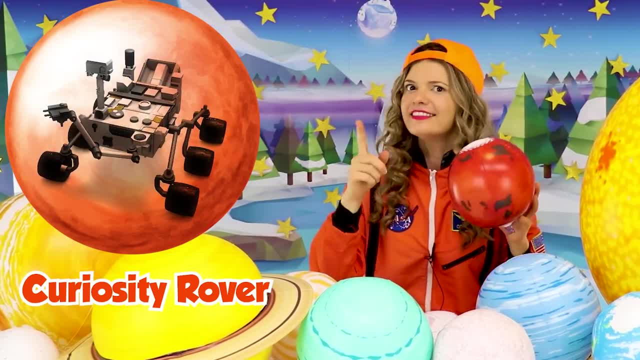 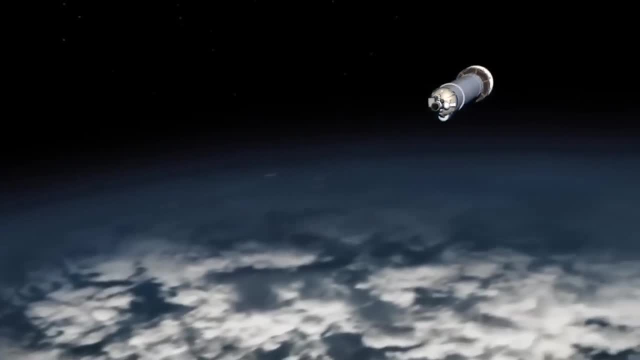 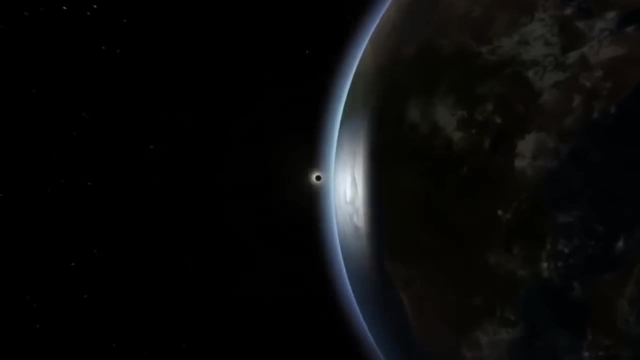 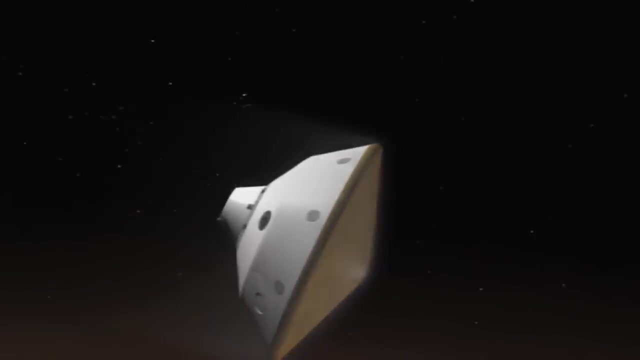 was sent to mars to help us learn, was sent to mars to help us learn about the red planet, about the red planet, about the red planet. let's see how curiosity, let's see how curiosity, let's see how curiosity got to mars. got to mars, got to mars.